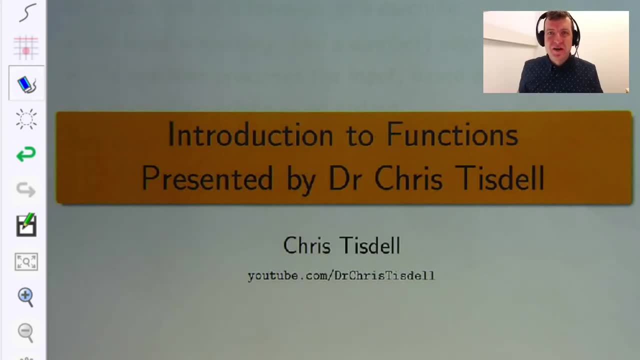 Now, in today's video, we are going to ask and answer the question: what is a function? Now, this is an introductory video aimed at people who might have done some mathematics at school, but they're certainly not experts, So they might be taking a Calculus 1 course. 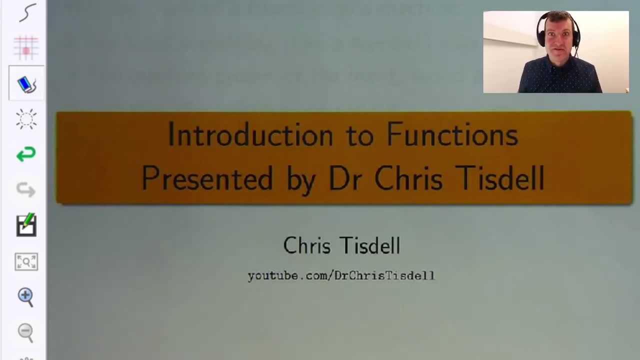 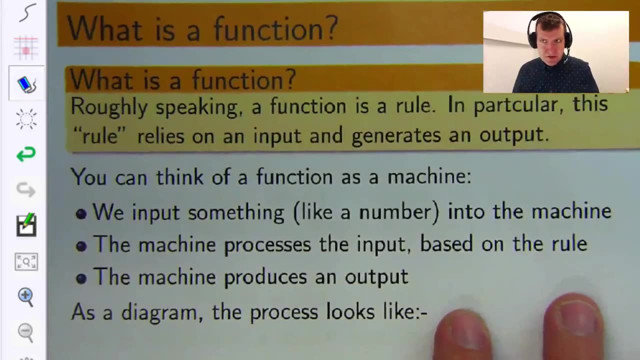 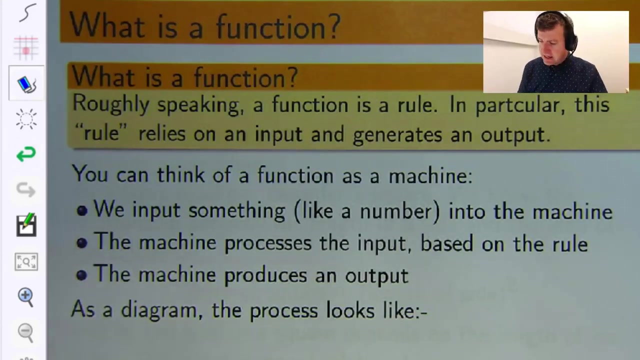 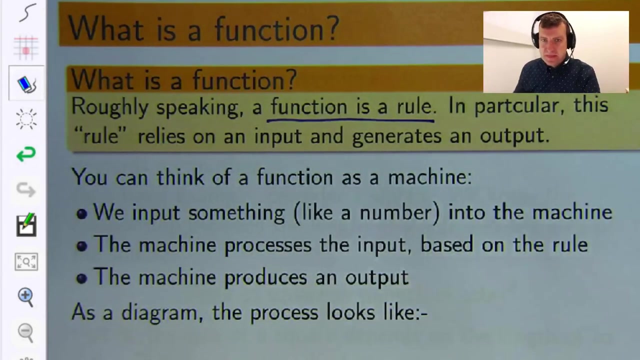 and the first thing you do with a course like that is talk about functions. So what is a function? Well, I'm glad you asked. Roughly speaking, a function is a rule. Now, in particular, the rule relies on an input and it goes to work. 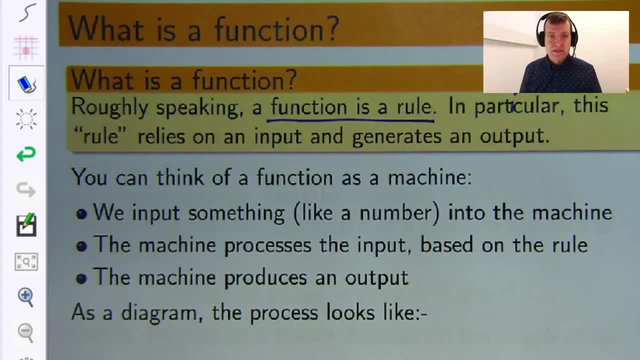 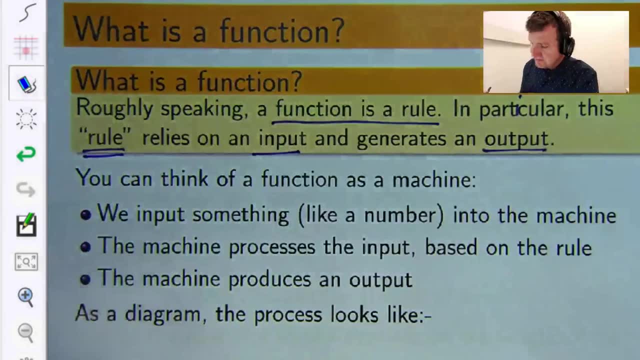 and then it spits out an output. So two important ideas there. There's the idea of a rule, there's an input and there's an output. So let me draw a little picture and give you an idea here. 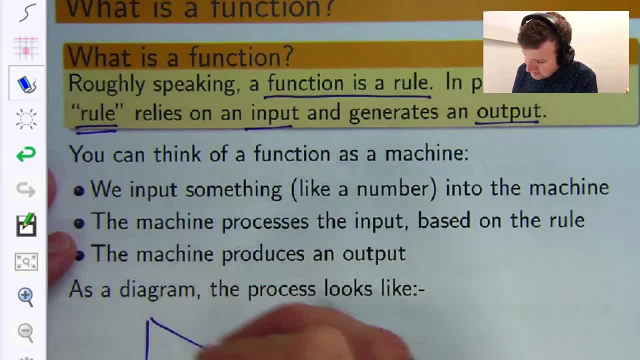 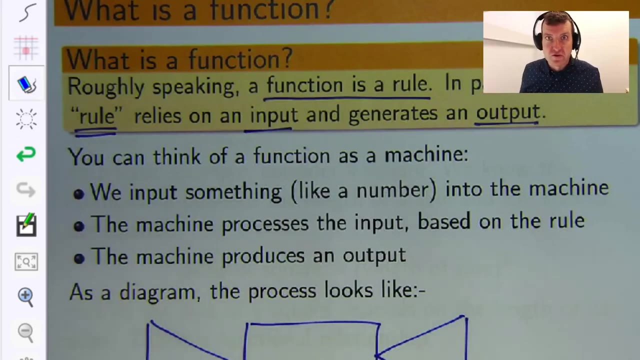 So if I was to draw a little picture here of what a function does, I can draw a little schematic kind of diagram here. Think of this as like a function machine. Our function is like a machine that follows a rule. I input something. 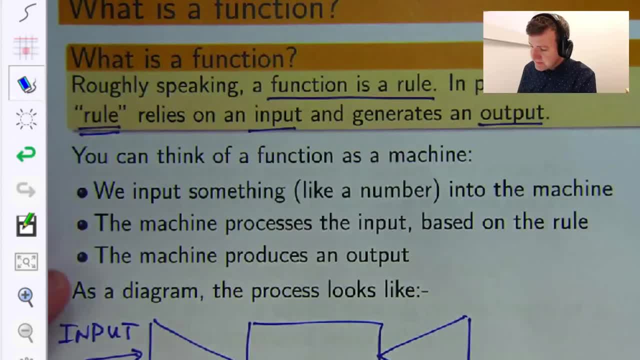 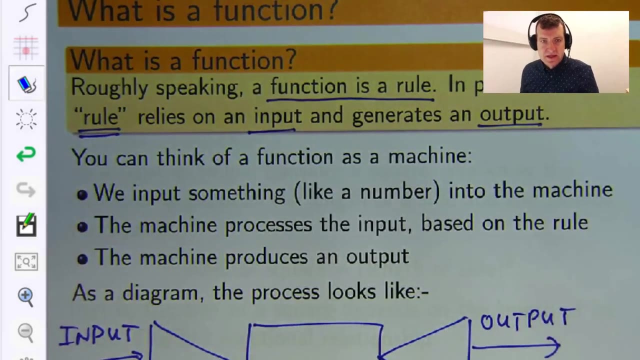 In mathematics, you input, I input a number, the machine goes to work according to a rule and it spits out something at the end after it's done its work. Okay Now, in mathematics, the inputs are usually numbers. 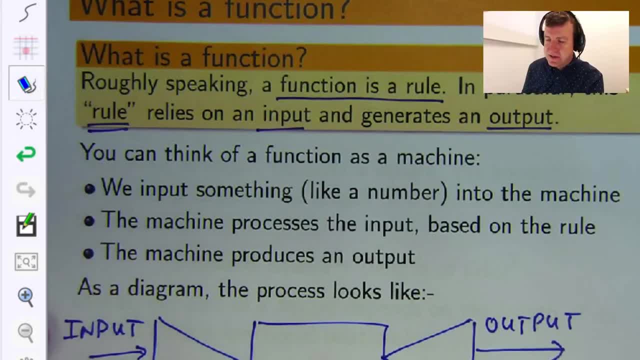 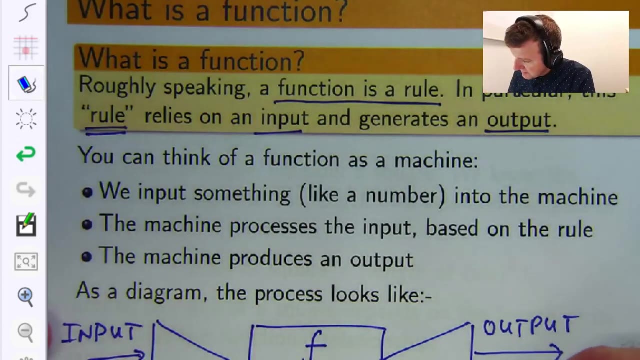 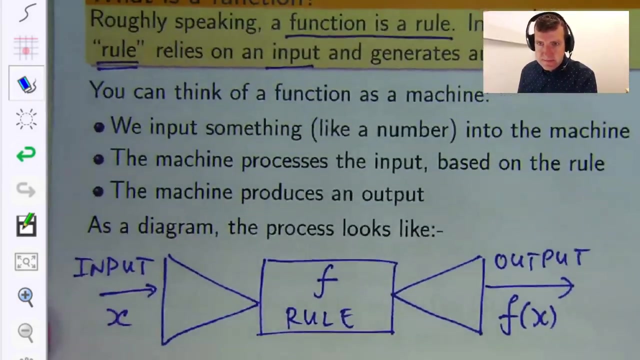 so 2 or 3 or pi or 100.. I'm going to write x just to denote just any number. The rule is usually denoted by some f and the output is written as f. Okay, so let me just move that up a bit. 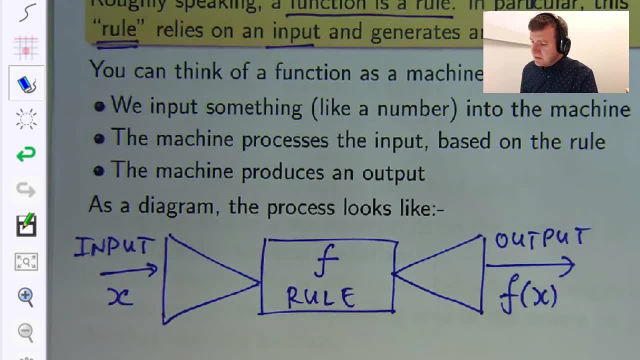 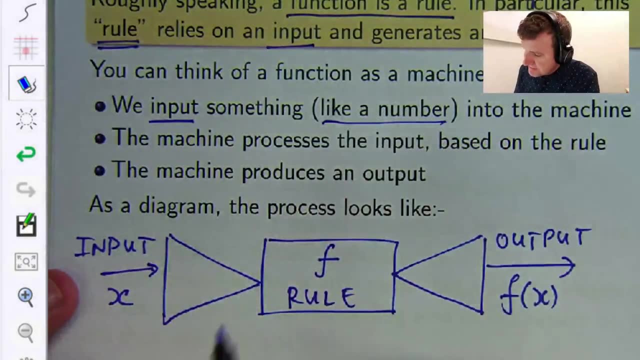 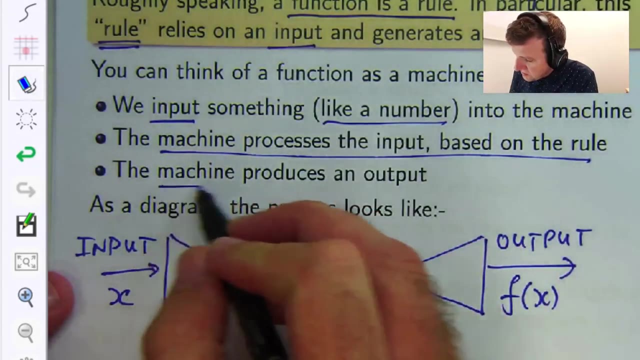 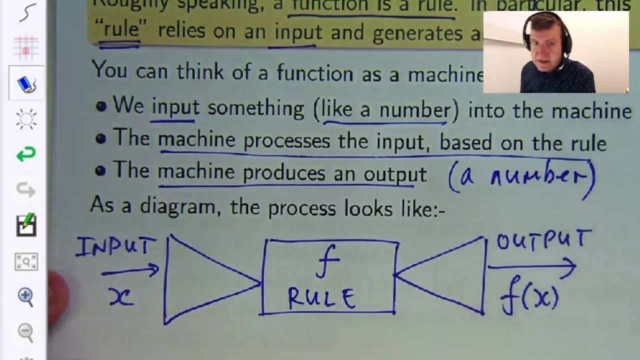 Okay. So let me just repeat that We input something into the machine, something like a number, The machine processes the input based on the rule and then you, the machine, spits out an output, Again a number. Okay, 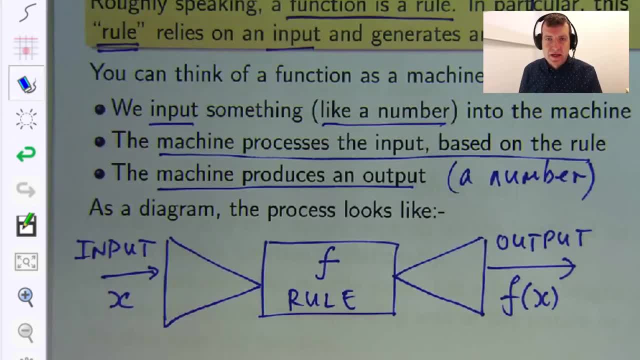 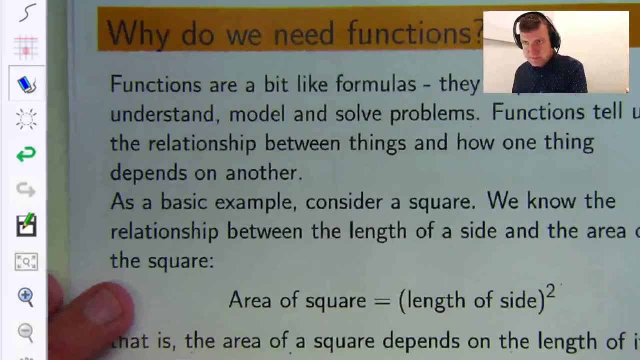 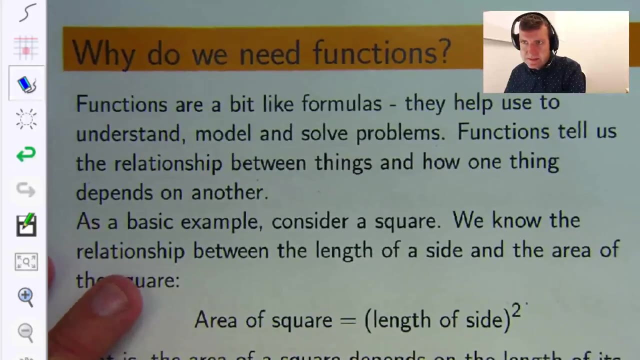 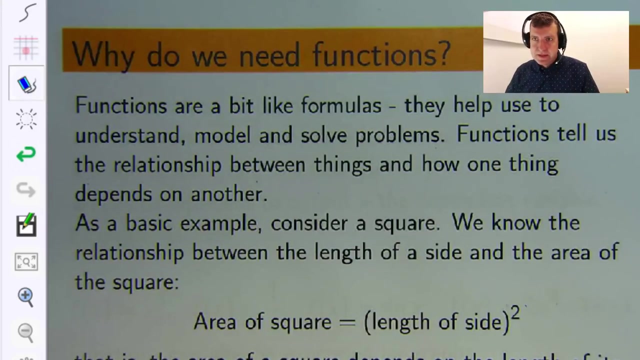 So that's how a function works. Now, why are functions important? Why do we need functions? Well, I'm glad you asked Why do we need functions. Functions are a bit like formulas: They help us to understand model. 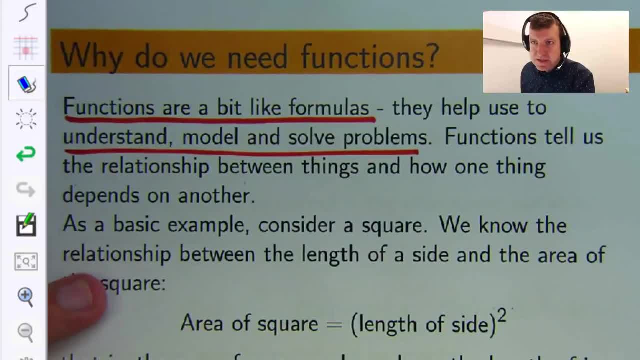 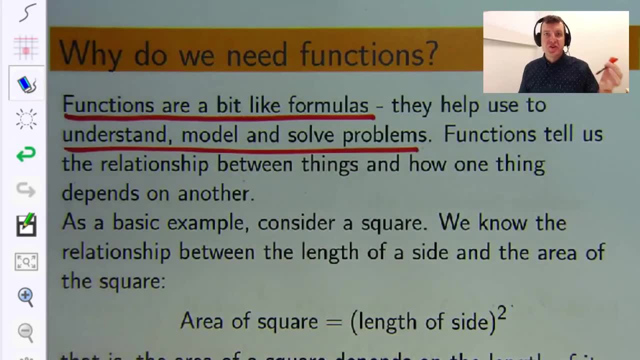 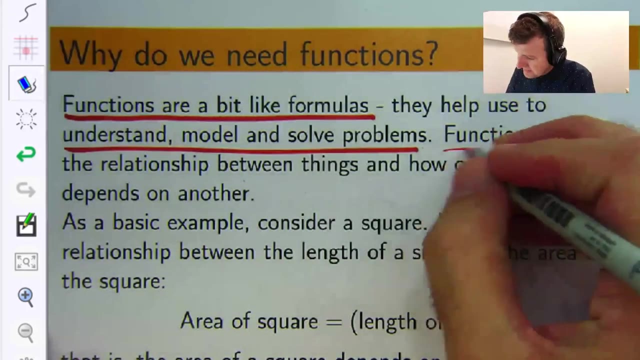 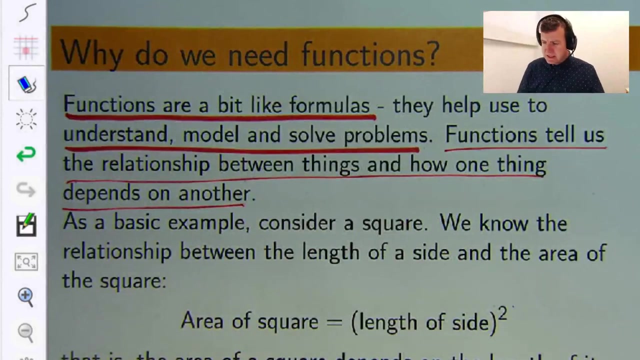 and to solve problems And, in particular, functions tell us how one thing depends on another thing, Okay, Okay. So let me unpack that a bit more and I'll do a little example here. Suppose I've got a square and we want to. 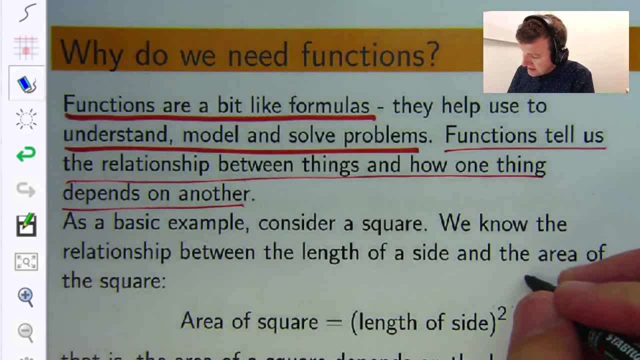 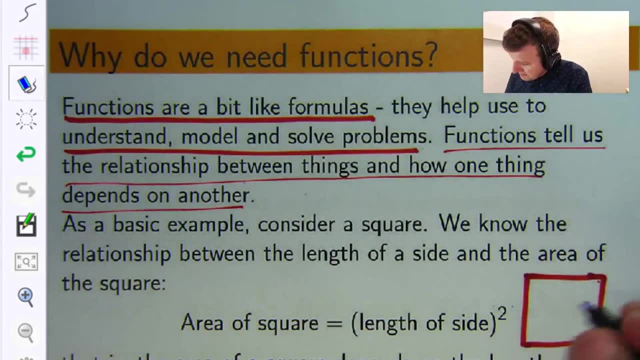 compute the area of a square. Now, we all know that from basic school. Here's my square. To compute the area of a square, you just take the length of one side and you square it. Okay, So if this is my square, 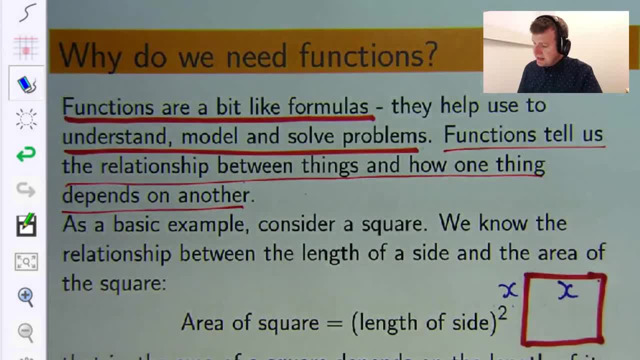 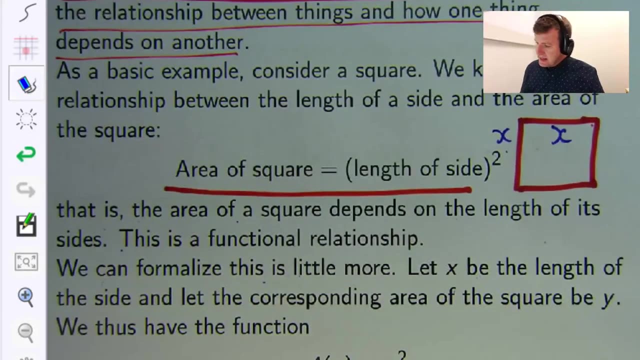 I might have a side of x and x, The area of the square would be x squared. Okay, So this is our basic starting block, And the area of a square depends on the length of its side. So as the sides increase. 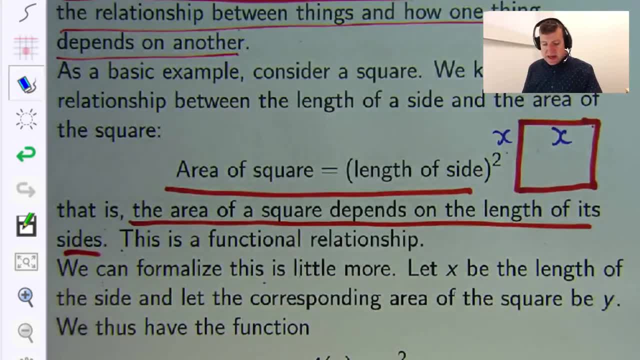 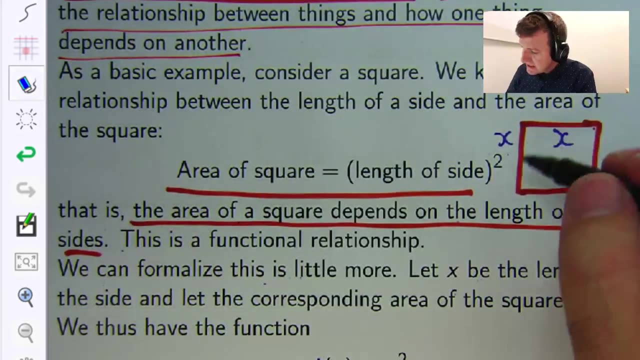 the area will also increase. Okay, Now we can formalize this mathematically a little more. Let's do that If I, as in this diagram, I let x be the length of the side and let the corresponding area of the square 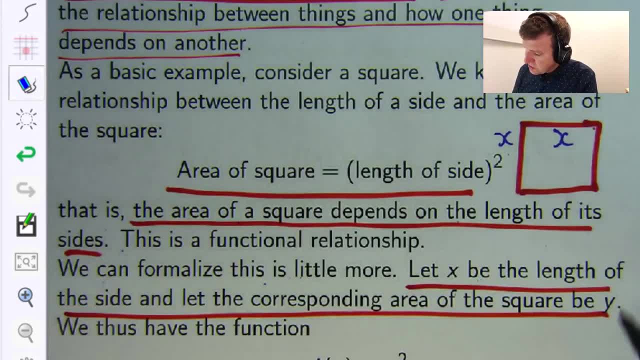 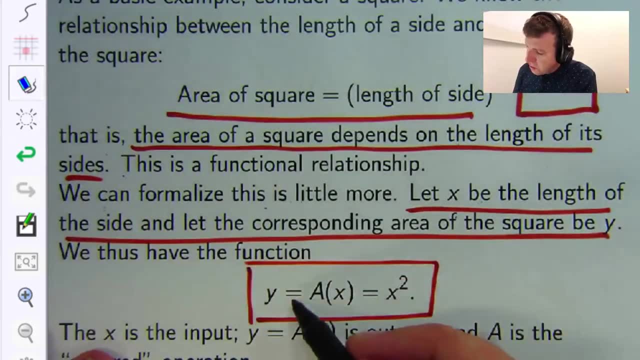 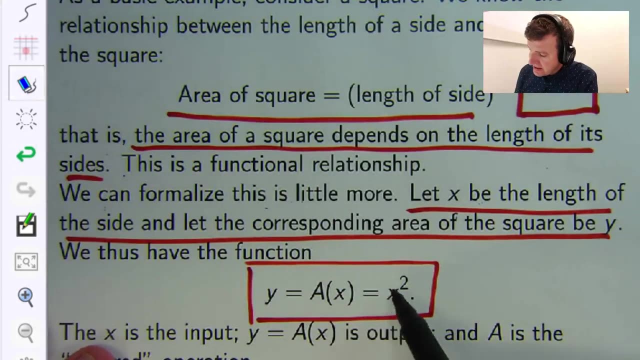 be the length of the side, The area of the square be y. Now we can write the function: y equals, say, a of x. I haven't used f here, I've used a for area And the area is just x squared. 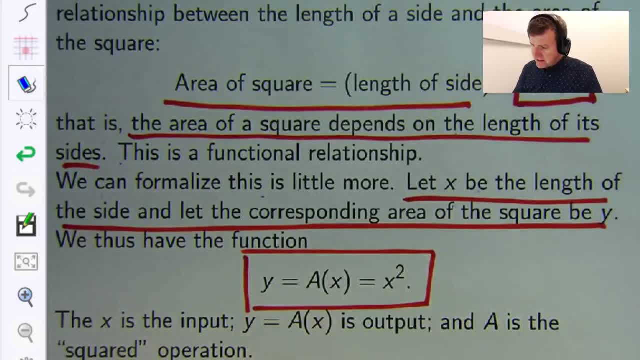 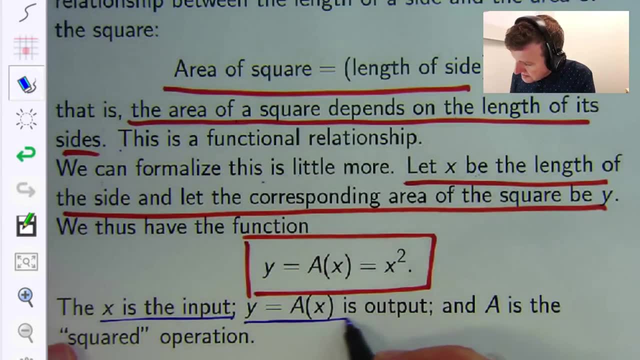 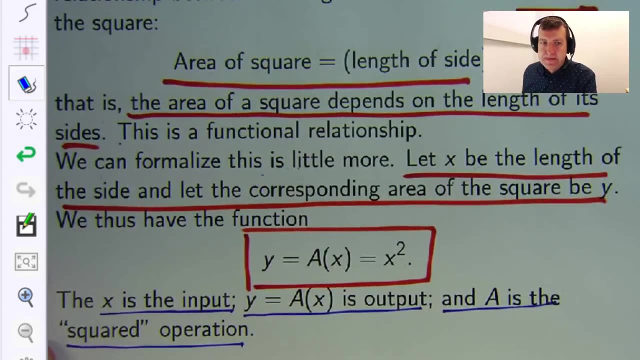 So how does this relate back to what we did on the previous slide? Well, x is the input, y equals a of x is the output and a is the squared operation. Okay, So imagine I was. I had a square with side equal to 2 units. 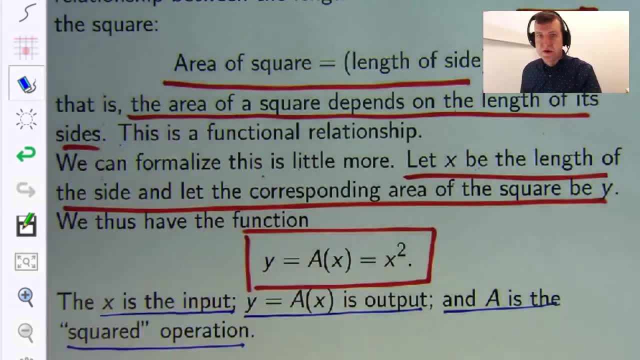 I would put in 2 into my squared function. The squared function squares 2.. And the output you get is 4.. Okay, So that's how it works. And relating it back to a very, very simple example, Okay, 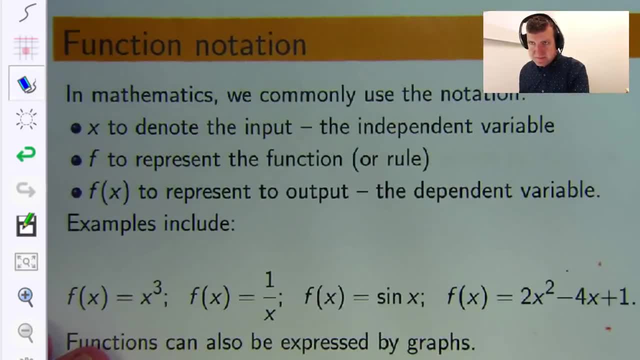 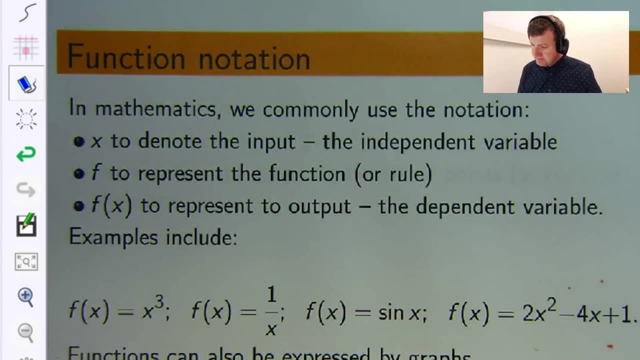 So that's a little bit about the need for functions. Here is how we can write functions. Well, down here we've got all sorts of functions. Okay, Now, these are written with the rule in mind. So here the rule is. 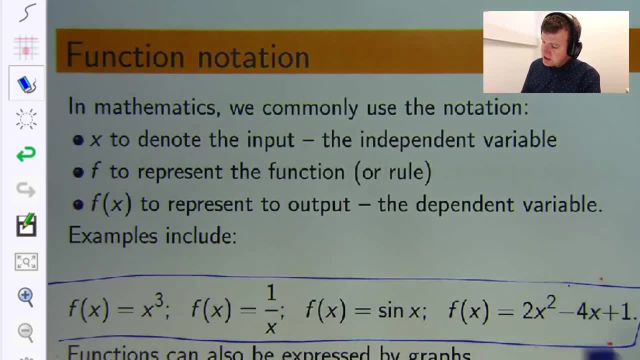 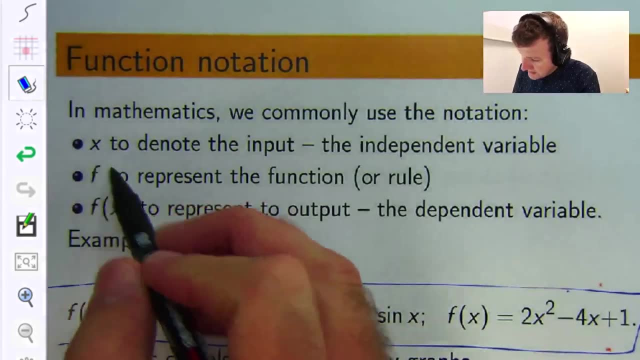 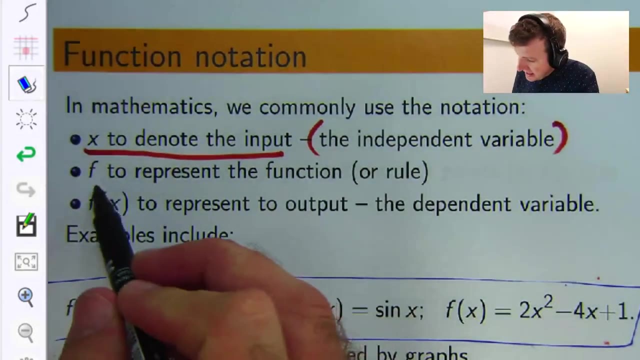 the cubic rule. Here you invert, Here's the sine function And here is some sort of quadratic or polynomial. Now, usually what we do is we use a notation x to denote the input. The independent variable f represents the function or the rule. 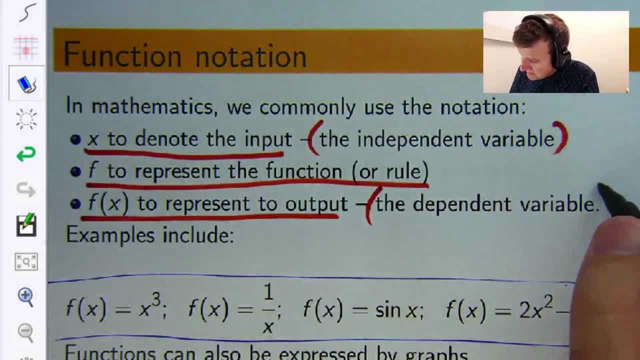 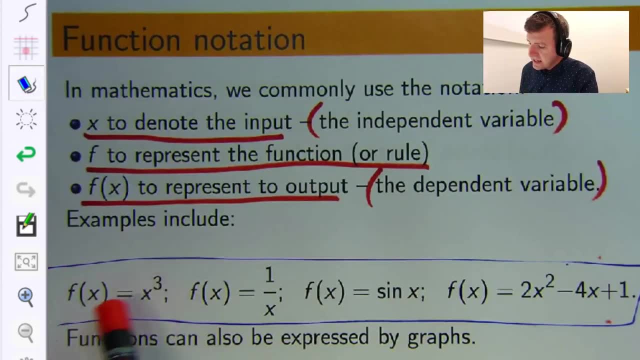 And f of x represents the output, The dependent variable. Okay, And this is the usual notation that we use. So here you might think: oh no, the function's x cubed. Well, actually, really speaking, the function is just the cube. 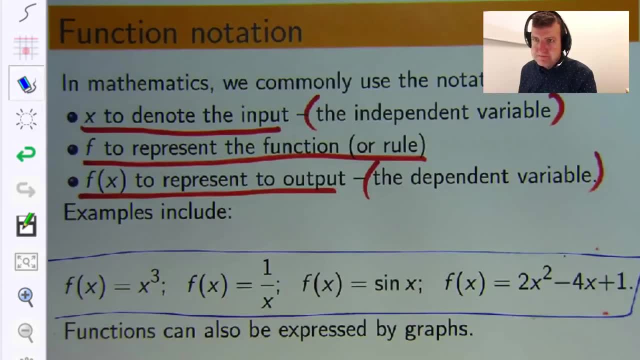 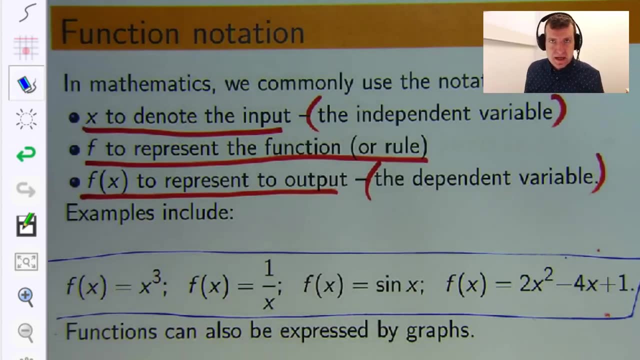 Okay, Now another really handy way of expressing graphs and writing graphs is through pictures, And pictures are awesome because they convey a lot of information in a visual, understandable way. So, for example, let's take this first graph, the first function. 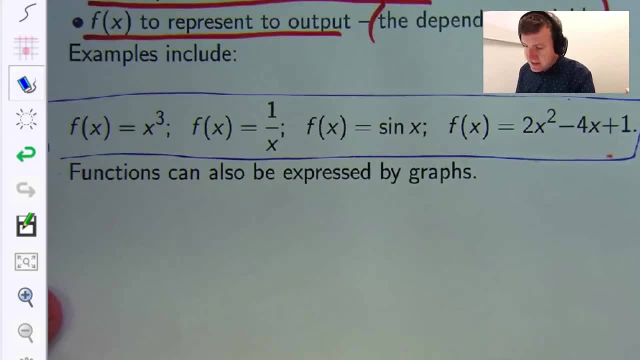 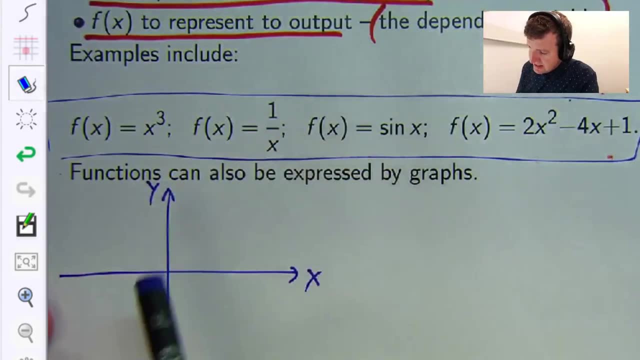 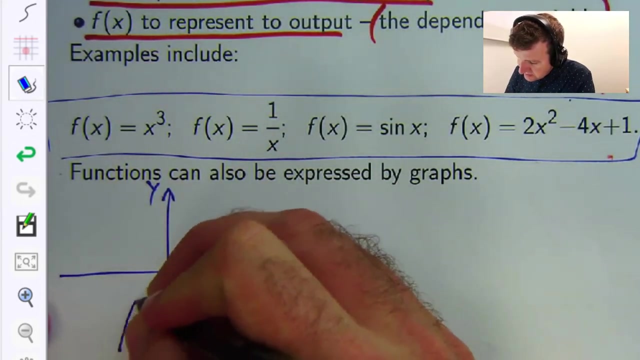 and see if we can draw it in as a graph. So if I draw some axes in, Okay, I've got the horizontal axis as the x-axis And the vertical axis as the y-axis. If I was to plot x cubed, it would look. 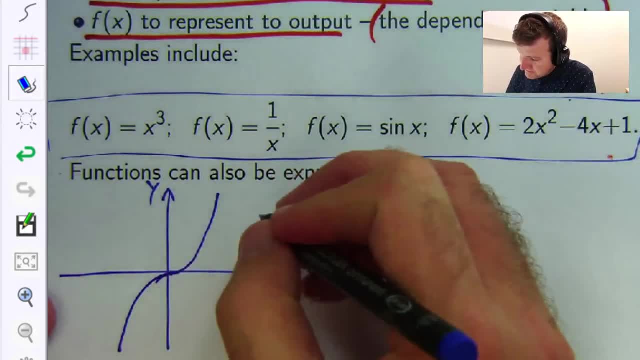 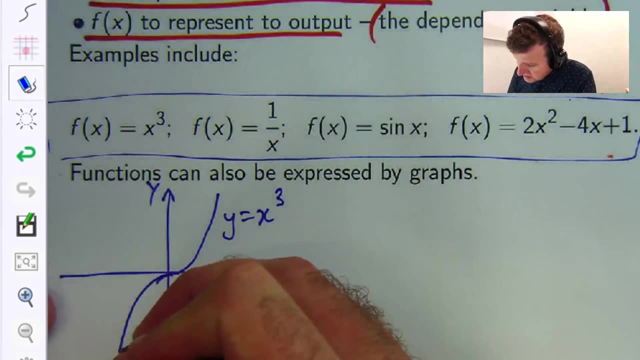 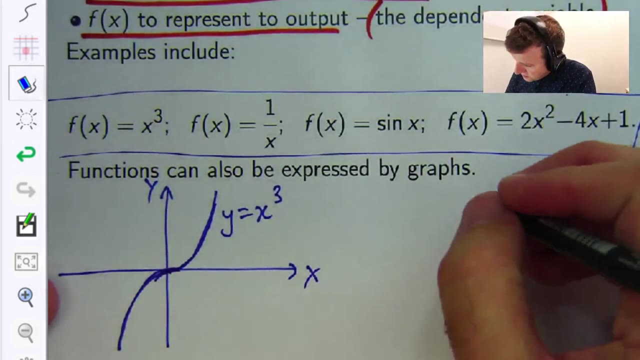 something like this: Okay, And I'll put y equals x, cubed in there. So in this graph, for each x point there's a corresponding y point, 1 on x. Again, let's draw in our axes 1 on x would sort of look like this: 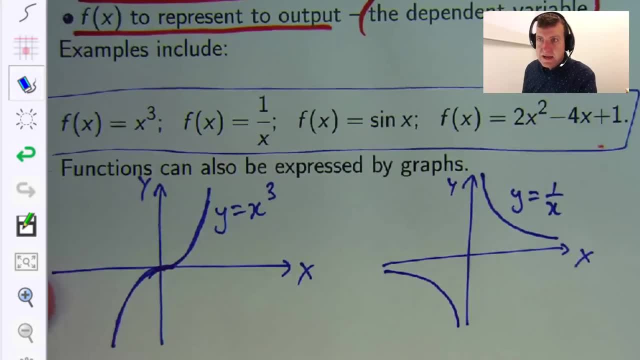 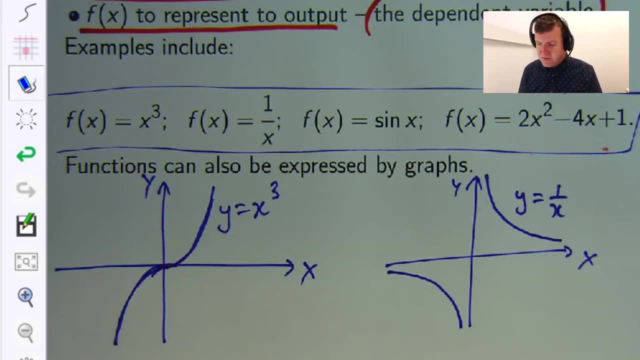 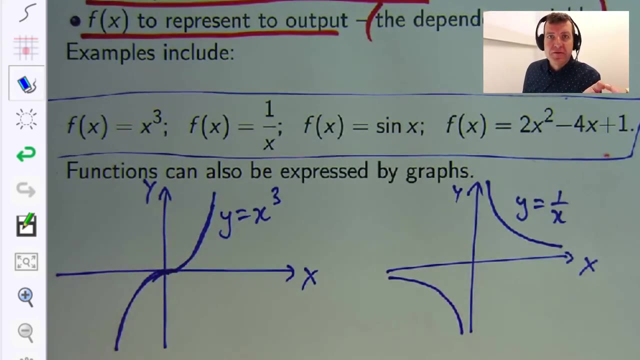 Okay Now, graphs are great because they convey lots of information in a visual way, So they're really brilliant ways, And we'll look at how to sketch these graphs in due course, But if you are stuck, if you want to look like, find out. 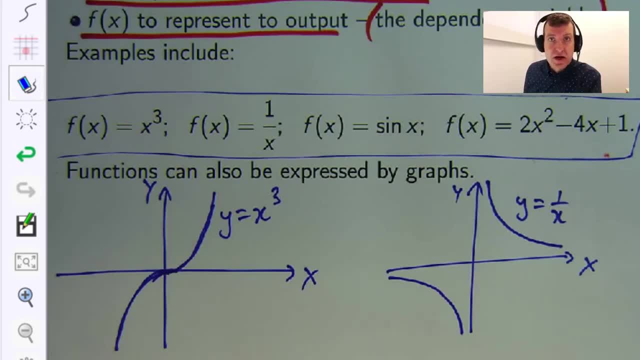 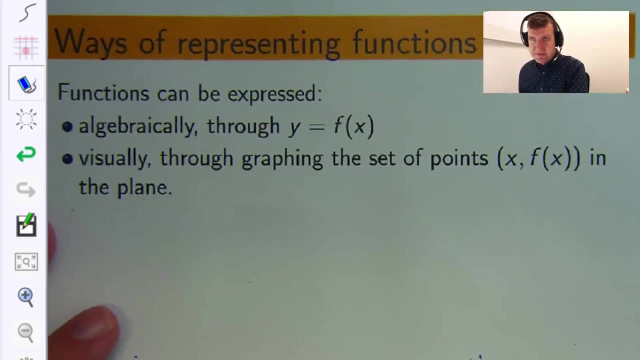 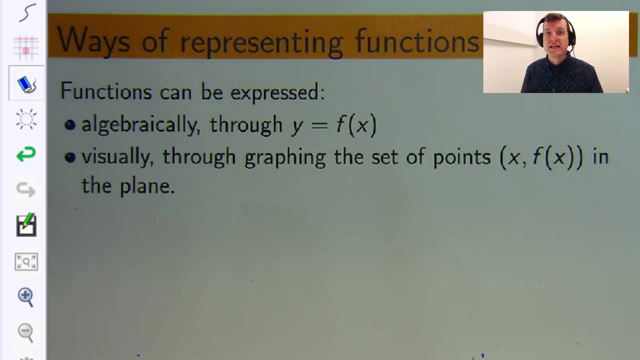 what a function looks like graphically. go to Google and type in x- cubed, and it will give you some pictures. Okay, So just to recap, Functions are important because they help us model and understand lots of different things, And, in particular, 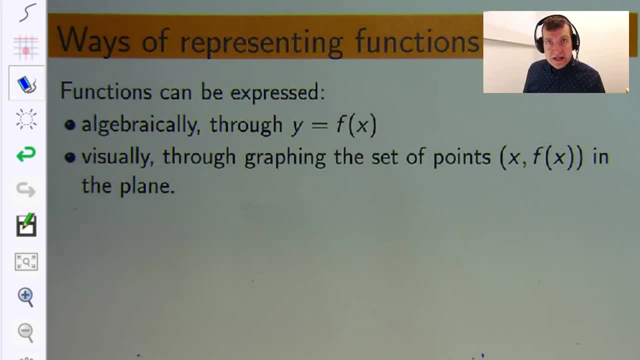 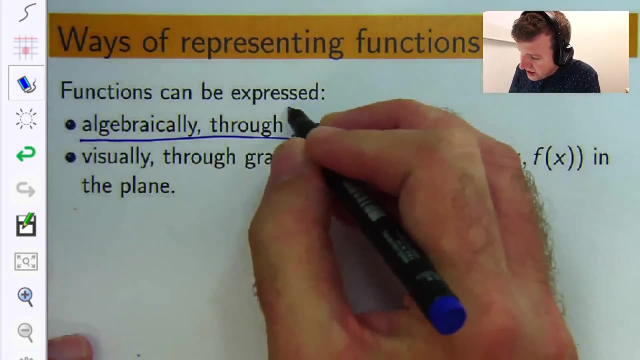 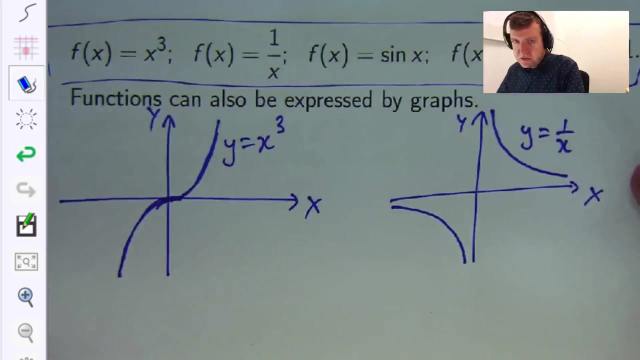 they help us understand how one thing depends on another thing. We can represent them in this y equals f of x form, Or we can represent them visually, So sort of moving on from these sort of graphs in the xy plus plane you might have. 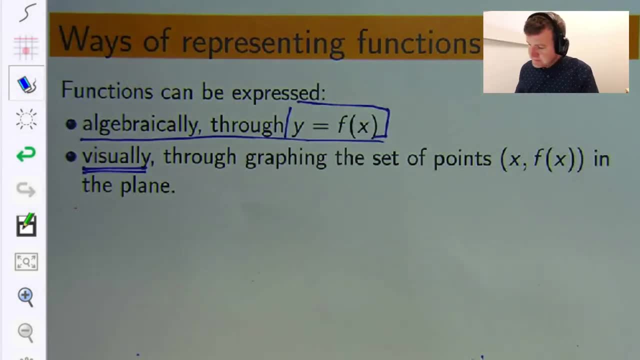 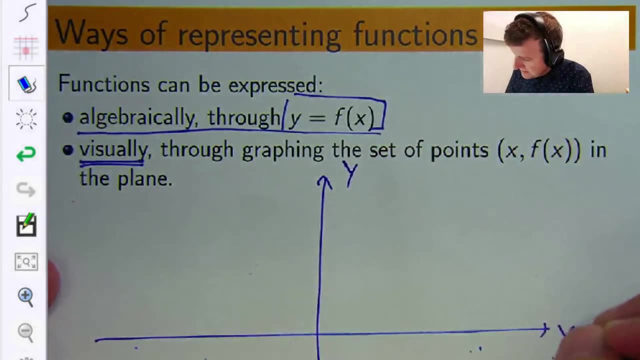 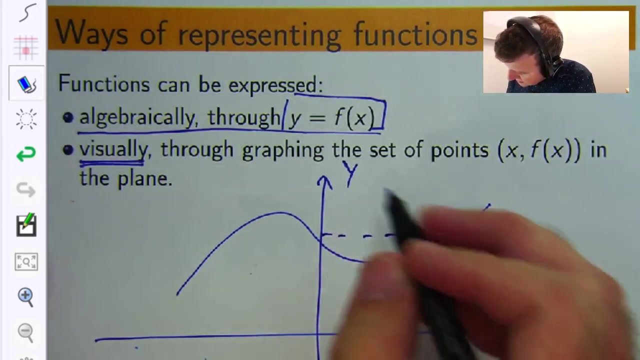 something like this: Okay, so let me just draw in a graph like that. Okay, that might be your graph or your curve, And for an x point on the x axis, in this case, there will be a corresponding y point on the y axis. 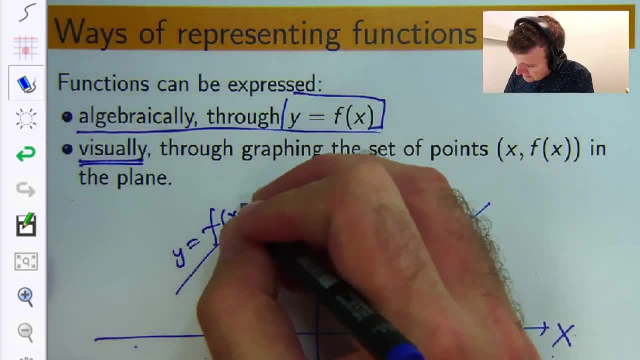 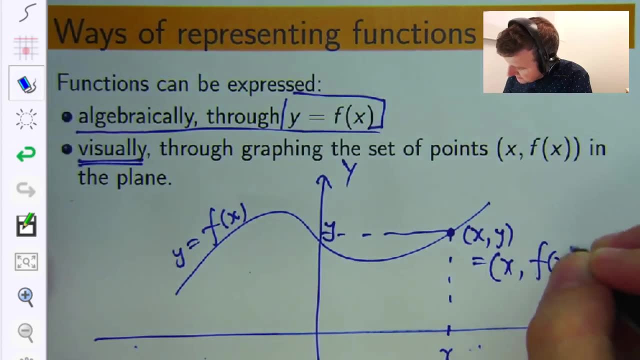 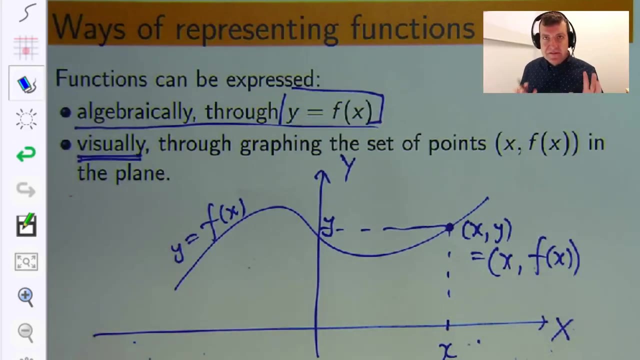 And this point here on the graph just has coordinates: x comma y or x comma f of x, depending on how you write it. Okay, functions are great. They are one of the basic building blocks of mathematics. They're really important because they help.